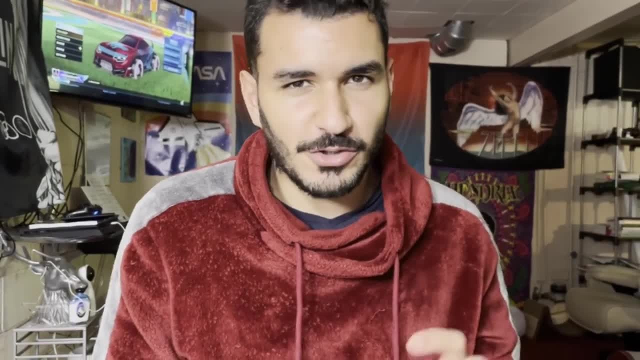 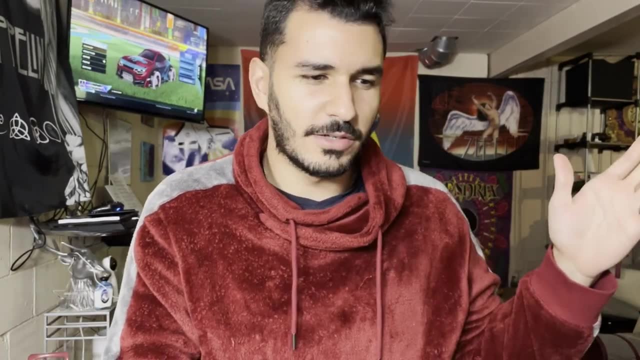 engineering just sounds cool, like if you go and tell anybody what kind of engineering you do, airspace is always the one that's like catchy or people are like, wow, that's so cool. so i'll be honest, that was probably one of the reasons. also is like, since everyone thought it was cool, i was 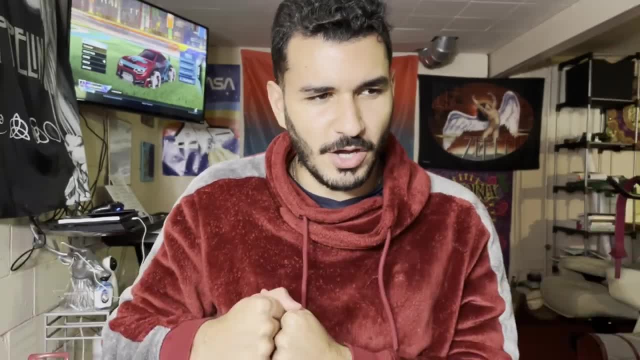 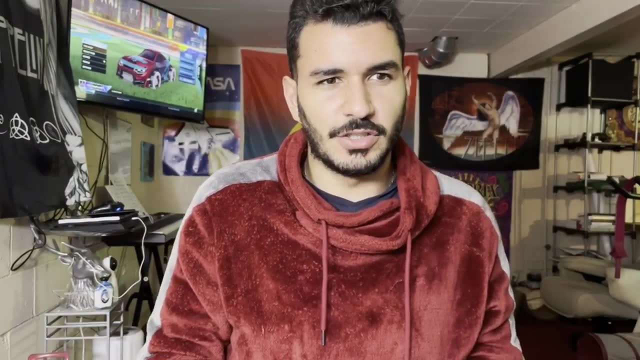 like okay, it must be like really nice. and as a naive freshman in college, my thought was that like okay, i'm gonna go into aerospace engineering, i'm just gonna design airplanes, like airplanes, like the whole thing. like i thought that basically as an aerospace engineer, everybody basically sits. 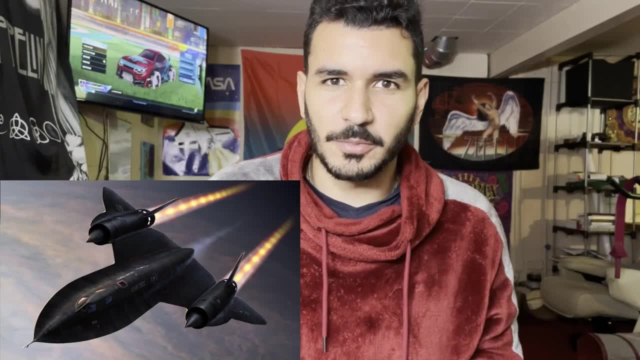 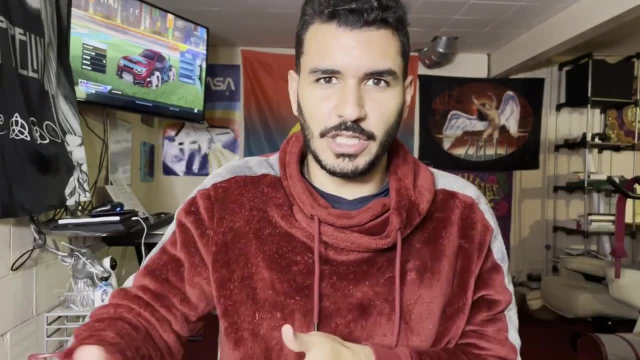 behind the computer and designs like the next generation, like sr71, blackbird. and i actually did take a cad design class during that semester where i was designing like an airplane wing and that was like super cool. but then when i looked at the curriculum and i looked at the classes, 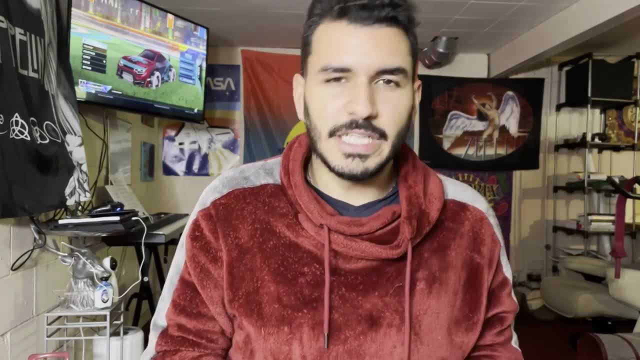 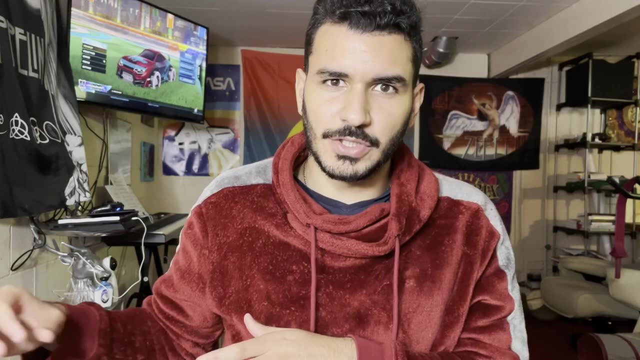 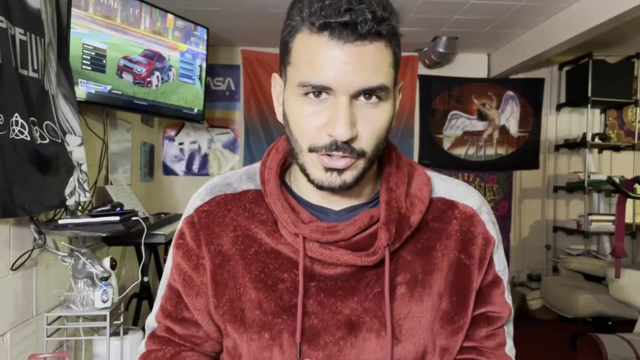 and i started seeing things like thermodynamics and gas dynamics and heat transfer and statics and dynamic systems and i immediately realized, oh my god, this is like mechanical engineering for like aerospace applications. like an aerospace engineering degree is essentially a mechanical engineering degree for the application of aerospace, so obviously you have like emphasis on aerodynamics and like 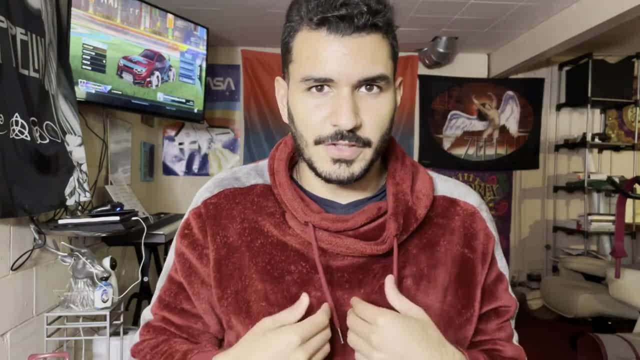 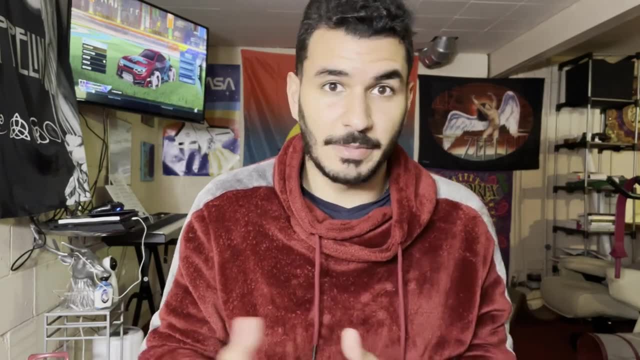 the forces that make an airplane fly and stay there. but at least at the university where i attended, most of the degree was still a mechanical engineering degree. you still took, i think, for the first three years this, almost the same classes as the mechanical engineers. and, in case you're, 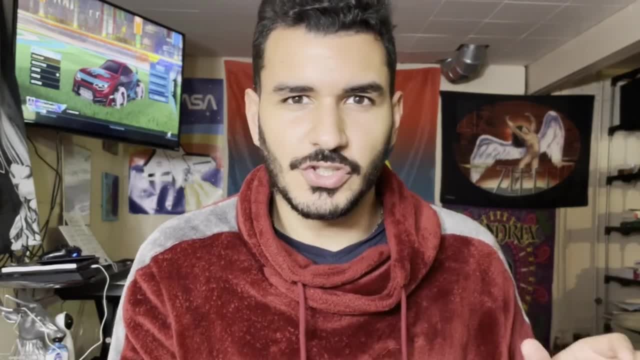 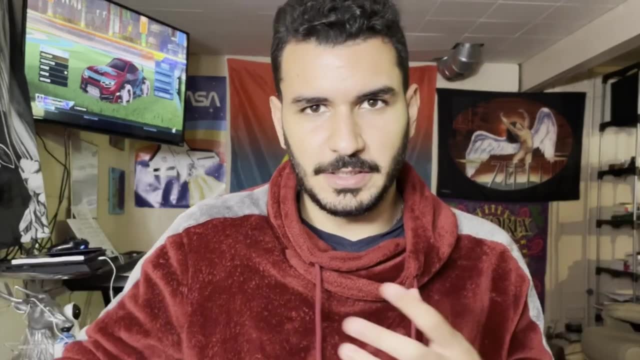 not aware. in my mechanical engineering video i talked about how i was not very interested in mechanics, like i'm a lot more interested in electromagnetics than i am in mechanics and anything mechanics related is not very exciting to me. so then again, after speaking to some of the professors and upperclassmen and getting a bit of a 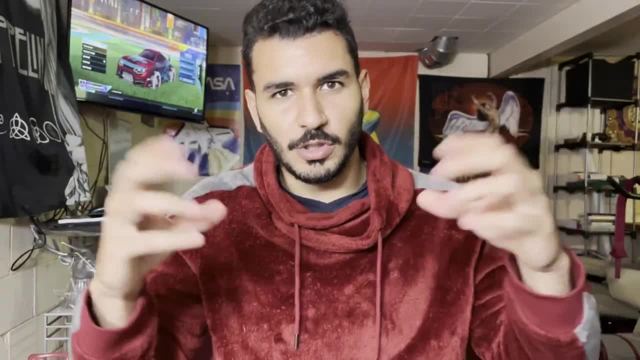 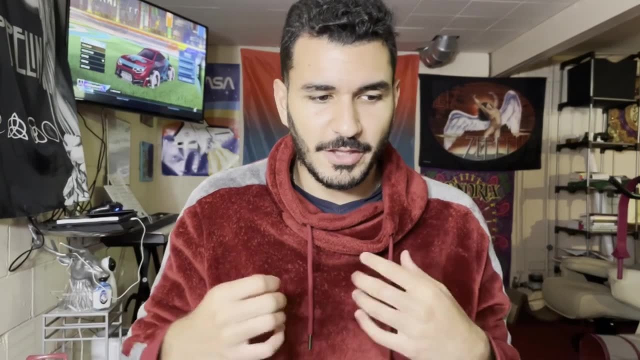 taste of what i would be doing. i quickly realized that, like airplanes, being cool and the desire to make an airplane look really cool is not really a good enough reason to study aerospace engineering. i mean, that's like nice to have, but i think you should also be very interested in mechanics. the 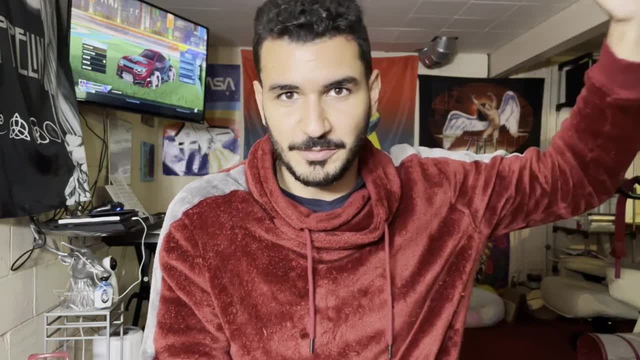 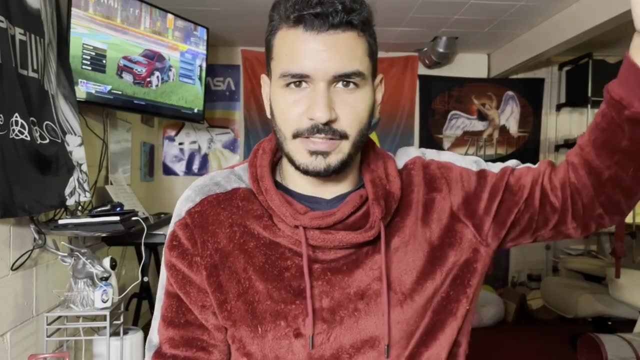 branch of physics that will help put the airplane in the air and maintain it and make sure it takes off and lands every time and make sure that the engines are doing their job. and make sure that the engines make sure that the propulsion system is doing its job, the airplane can take off the 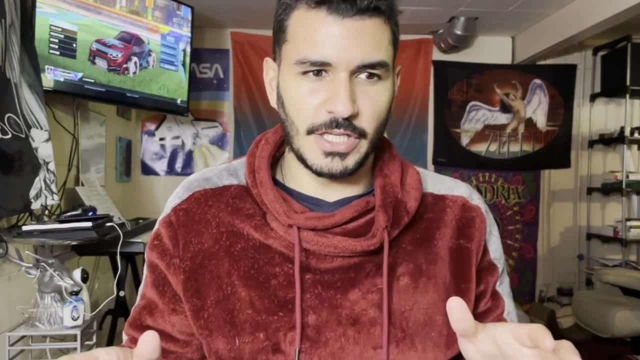 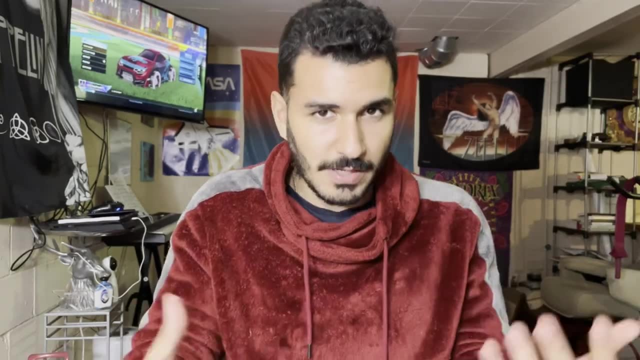 airplane can land. but the key idea i want you to take from here has nothing to do with aerospace or mechanical engineering or any of that. the idea is that i did the most amazing thing i could have done. i didn't realize at the time, which is i thought something was cool. i had an idea of what. 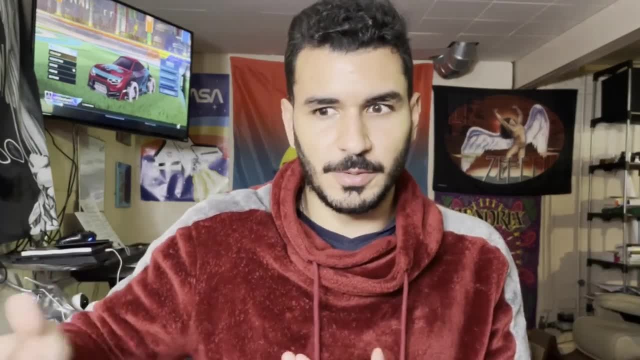 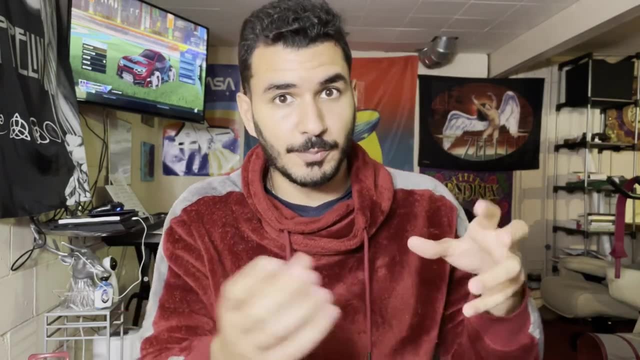 it would be and i just went and i tried it and i went and i took the classes, talked to the people, switched to the major and i learned from experience. i didn't just sit and like google all day. oh my god, what is aerospace engineering like? okay, that's a good place to get started, but then if you really